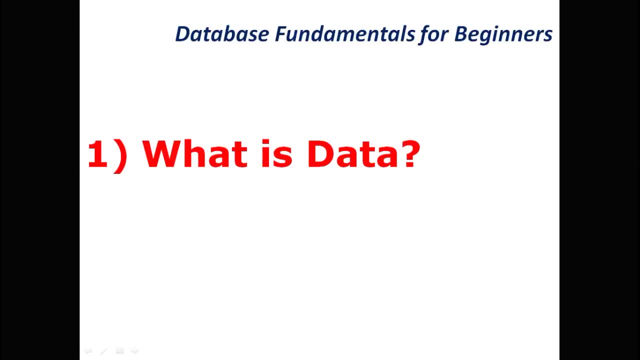 Next, what is database Database? It is collection of the data. which data? collection of related data. Next, what is DBMS database management system? It has different types. one is old, one hierarchical model, next network model, next latest one. 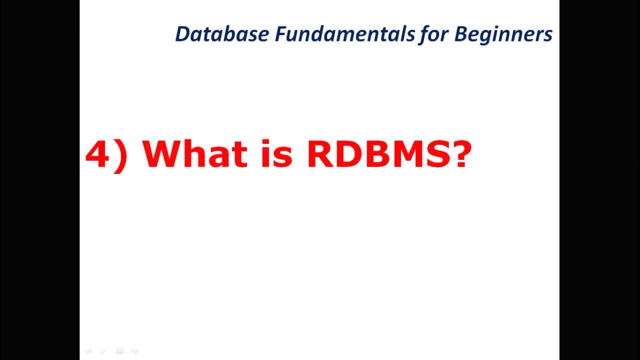 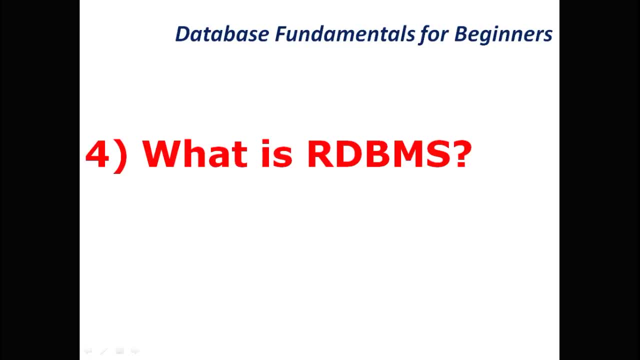 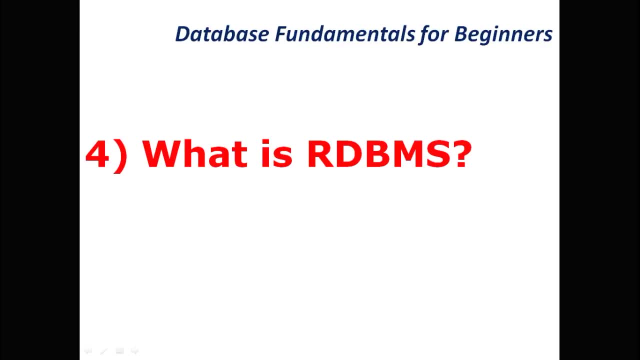 store or reference data. The most common database object is table. Other objects are indexes, stored procedures, views, sequences and many more. Next, what are the features of RDBMS? First one: data is stored in tables. Second one: 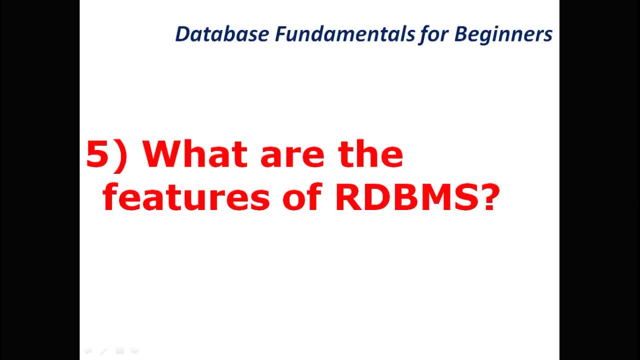 entire section of rows and columns will give only one value. Third one: relation among data is established logically. Fourth one: there are no physical links among data. Fifth one: there is no data redundancy. Sixth one: high security for data. Fifth one: data is 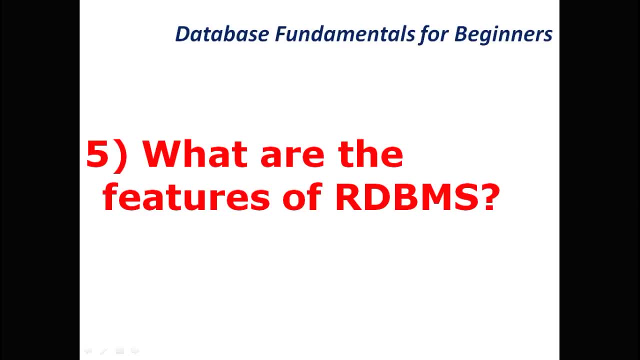 supported for data. Seventh one: it supports all type of data, Example numbers, characters and data, images, etc. Next, it supports null values. Next ninth one supports Cod rules C, O, D, D Cod rules. Next tenth one: it supports integrity constraints. Eleventh one: multiple users can access data. 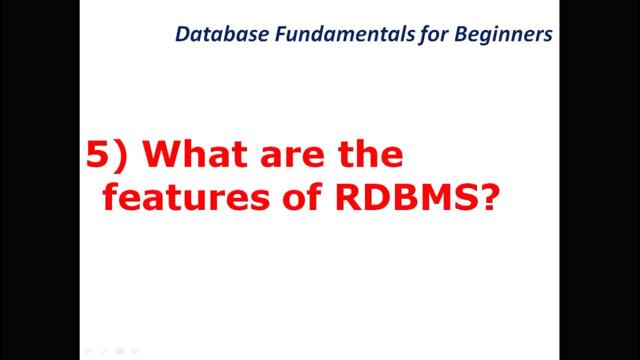 from any location. Next simple term: what is record? A record is nothing but collection of information or data. Next, what is table? Database table consists of rows and columns for storing set of records. Next main one: what is sql? Structured Query Language is used to secure records for every. 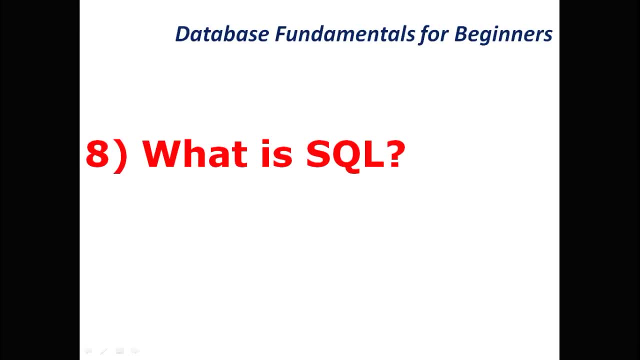 web data is used to communicate with a database. According to ANSI, it is the standard language for relational database management systems. Next, what is data definition language? DDL, SQL Structured Query Language- has three important subsets. What are the subsets of SQL? What are the? 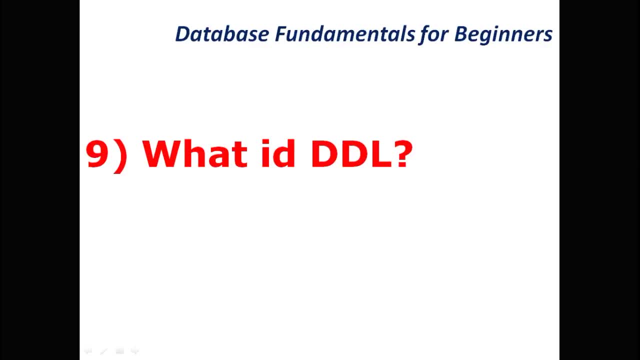 three important subsets of SQL. One is DDL- Data Definition Language. Second one is DML- Data Manipulation Language. Third one: Data Control Language, DCL. Now come to Data Definition Language. We already discussed it. It is a subset of SQL used to define the database structure. 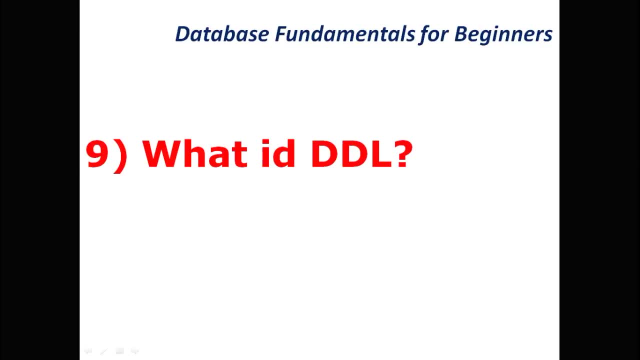 Important data definition. language commands are create. Create- To create objects in the database. ALTER Alters the structure of the database. DROP: Delete objects from the database. Truncate: Remove all records from a table, including all spaces allocated for the records are removed. 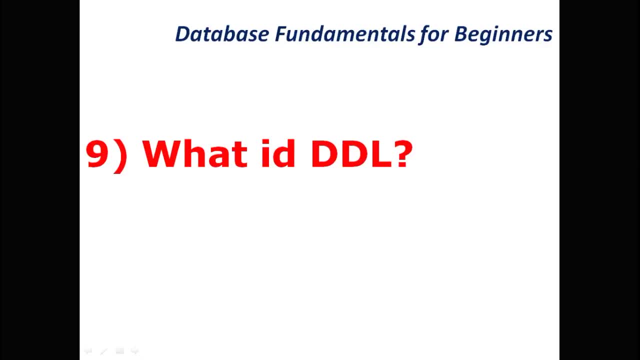 Next comment: add comments to the data dictionary. Rename: rename an object- Ok. next, what is data manipulation language, DML? It is also a subset of SQL used for managing data within schema objects. Important DML commands are select for software testing also. it is very important for retrieving data. 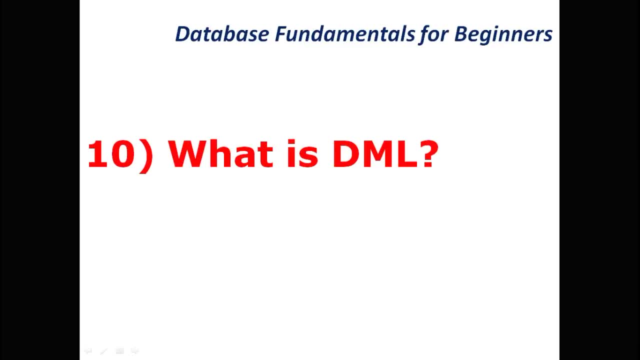 Select: We use select command for writing queries. We use select command for writing queries and sub-queries. Important DML commands are: one is select: retrieve data from a database Select. What is select: Retrieve data from a database Select. 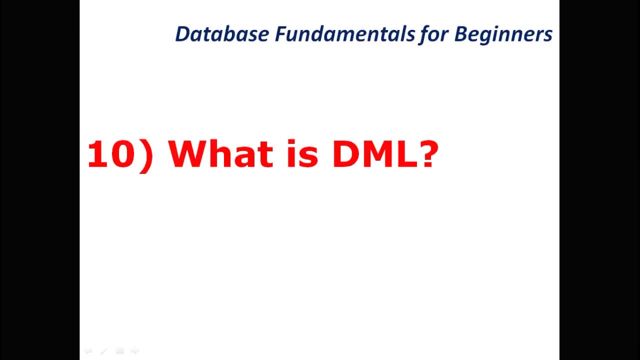 Next insert: insert data into a table. Update: updates existing data within a table. Delete: deletes all records from a table. The space for the records remain. Next merge offset operation. insert or update operation. Next call: call a PL, SQL or Java sub-program. 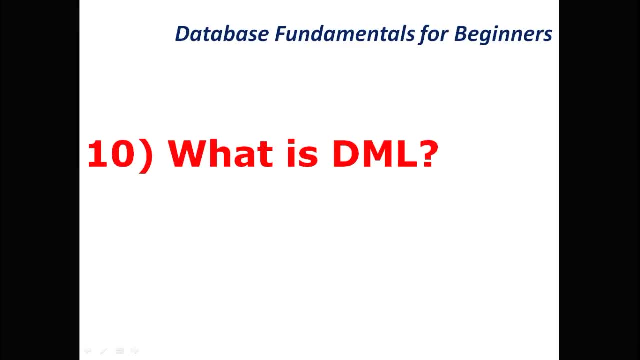 This call is not for all RDBMSs, Ok. here, important are: select, insert, update, delete, Ok enough. Next, what is data control language? DCL? It is also a subset of SQL used to control the data. 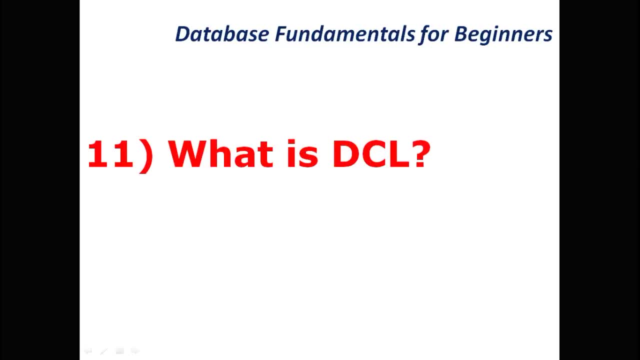 Important DCL commands are: grant: gives user access privileges to database. Next, revoke: withdraw access privileges given with the grant command. Ok. Next, what are the important RDBMSs that use SQL? Important one: What are the important RDBMSs that use SQL? 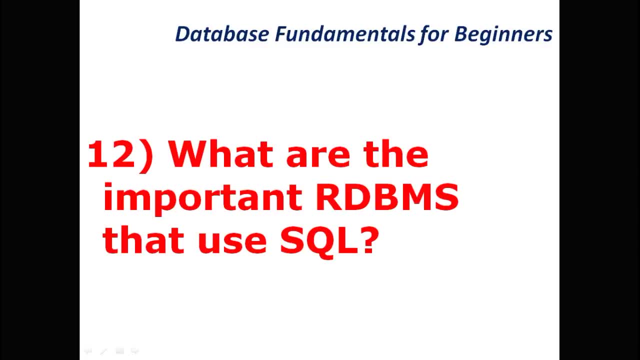 Important relational database management systems that use SQL are: Oracle, MySQL- Ok. MySQL. Microsoft SQL Server, Sybase, DB2, etc. Top three: Oracle, MS, SQL Server, MySQL- Ok. Next, what is SQL Server? SQL Server is a relational database management system developed by Microsoft. 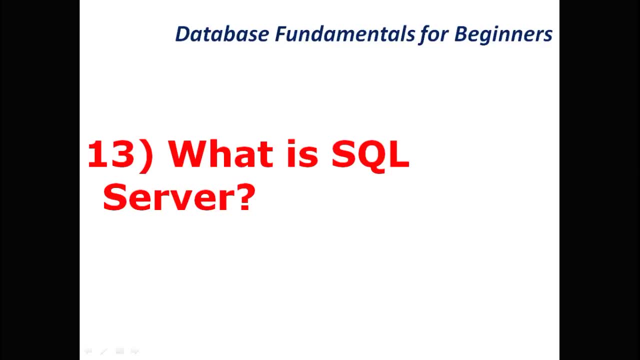 SQL Server runs on TSQL, Transact SQL, a set of programming extensions from Sybase and Microsoft that added several features to standard SQL, including transaction control, exception and error handling, row processing and declared variables. Final conclusion: SQL Server is a relational database management system developed by Microsoft. 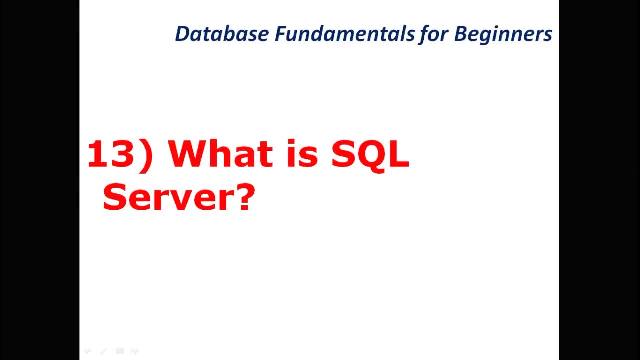 It is commercial RDBMS In this MS SQL Server free version also there for small scale organizations. MS SQL Server express edition. MS SQL Server is MS SQL Server is commercial software, But in this we have free versions. also Free version is MS SQL Server express edition. 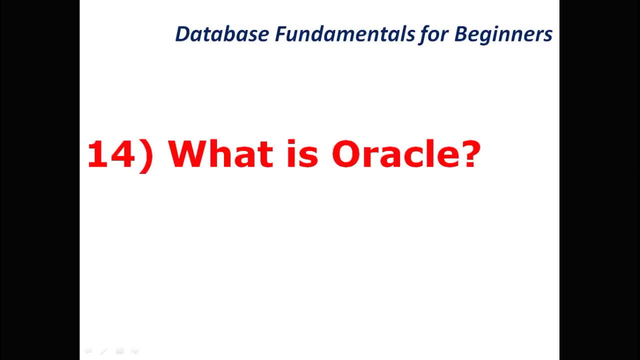 Ok, Next, what is Oracle? The Oracle database, or Oracle RDBMS, is an object to a relational database management system. Oracle database is an object to a relational database management system- O, R, D, B, M S, Developed and marketed by Oracle Corporation. 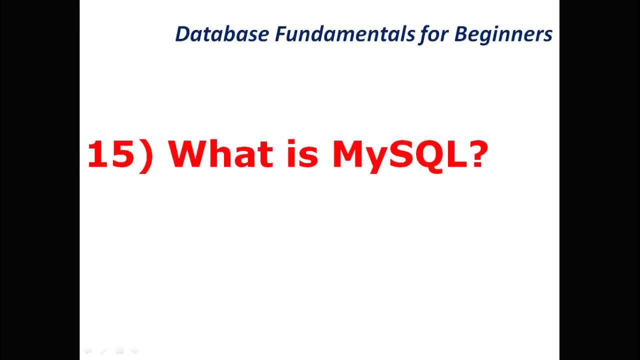 Ok, Next, what is MySQL? MySQL is an open source relational database management system. It is very fast, reliable and flexible database management system. Actually, it is open source- open source, But in this MySQL we have commercial software also. If you want more features and technical support, they have commercial software. 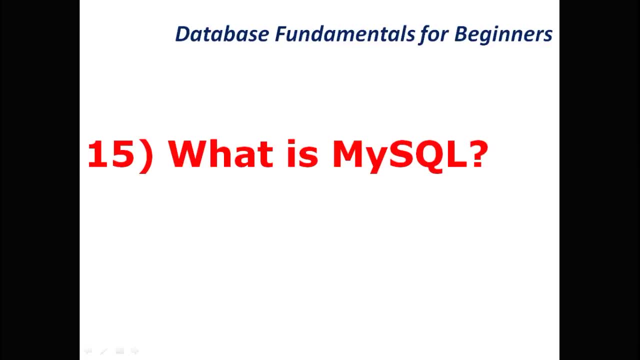 also See already we discussed: MS SQL Server is commercial software, but free edition. also there SQL Server express edition. Next, MySQL is open source, Open source software, but in this we have one or two paid versions also. Basically MySQL is open source. 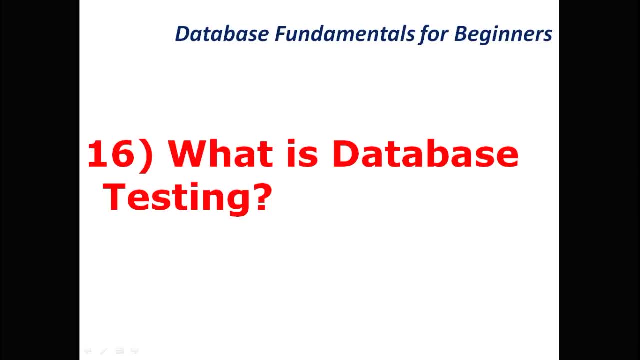 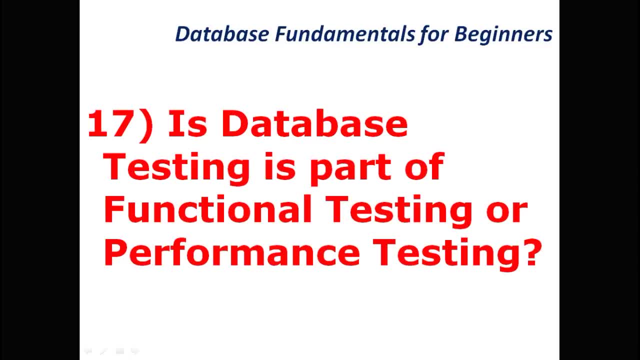 Animating there many and sharing. Verifying pragmatic, emotional self-management. Regular megabanks and collaboratorial interact drowsiness. Verifying all means of operation: social, financial and Also owners of professional ud scarifying faces circumstances, programs. Verifying 어떡ua metrics and surgical execution. Verifying procedures needed for the practice. What we can learn from this course. Verifying of dashboards in a data Soul трав activities. Verifying or counting which Indonesian first-iele landmark. 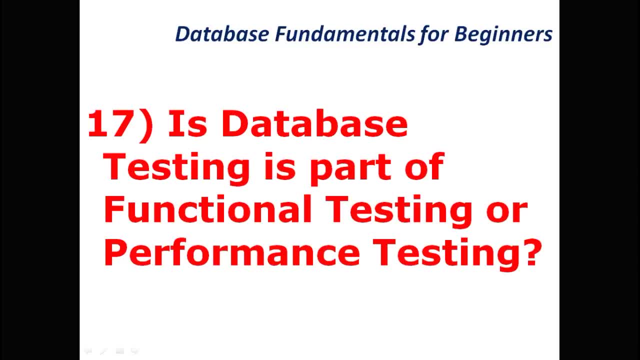 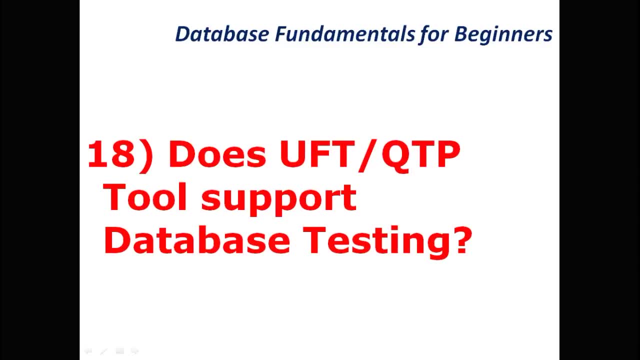 Database testing is subset of functional testing and subset of performance testing. Does UFT- formerly QTP- support database testing? Yes, UFT has integrated MS Access database engine. It supports SQL. And one more thing: in UFT we can use built-in feature data table for conducting database. 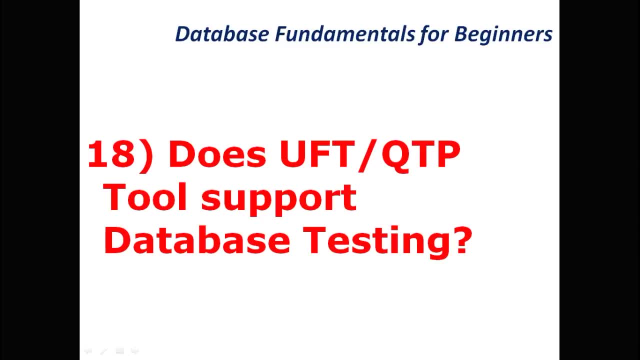 testing, Otherwise VBScript. VBScript feature features database objects, database connection object, database record, set object, etc. Using VBScript database objects also, we can conduct database testing in UFT, formerly QTP. Next, does Selenium support database testing? 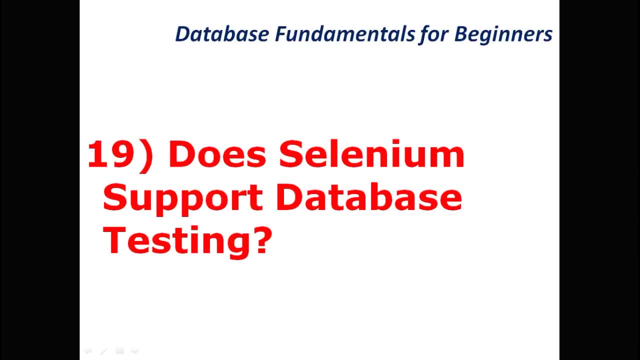 Yes, with the support of programming we can connect to databases and conduct database testing. See for Selenium. we can use either Java or Perl, or Python or Ruby or C-Sharp dot net, Next PC, Next Then PHP. 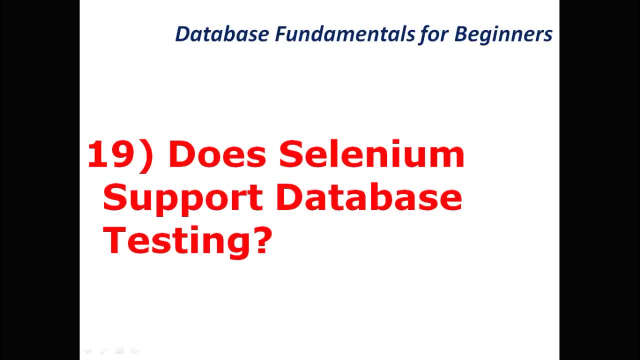 It supports six programming languages. We can use any one of those languages. If you use any language, for example Java, using Java programming we can connect to databases and conduct database testing. See Selenium supports database testing. Next UFT, formerly QTP. 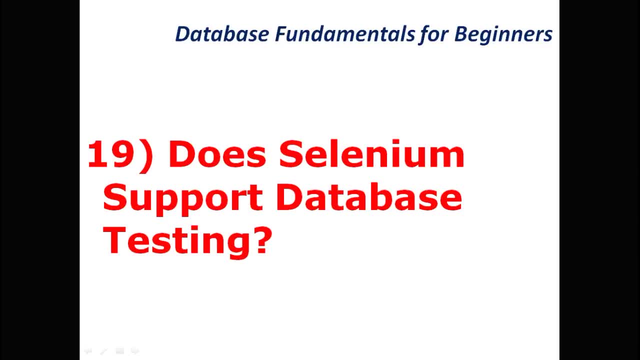 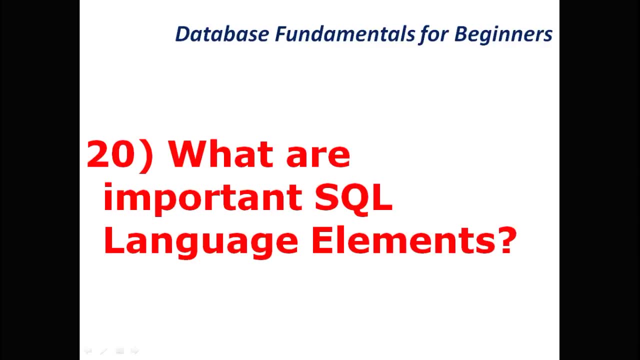 Similarly, QTP supports database testing. Next, What are important SQL language elements? One is: identifiers: names of objects such as tables, views, columns, databases and servers. identifiers- Second one: data types define the types of data that are contained by data objects, such 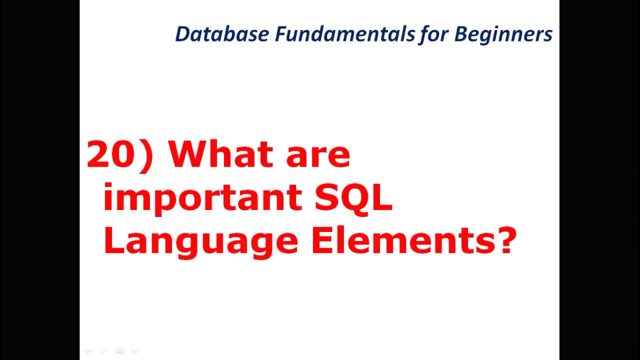 as columns, variables and parameters. Next, What are important SQL language elements? Second one: data types. Third one: constants: symbols that represent specific data types. Next, fourth one: operators used for conducting mathematical comparison and logical operations. 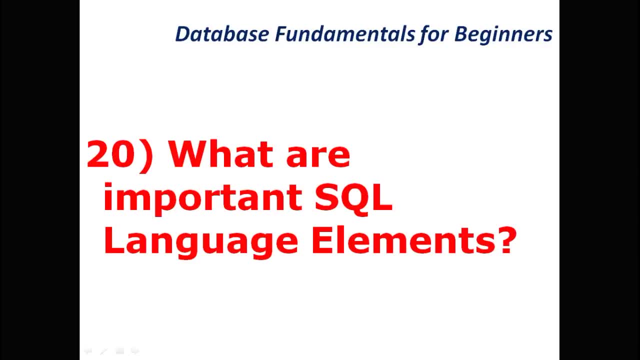 Next, One line of data, also inside the document that help you to understand the eyeball, as does one line of data. Next, One line of data uses a function that can be historians use to rewrite a table for row and table for drop in upside down. 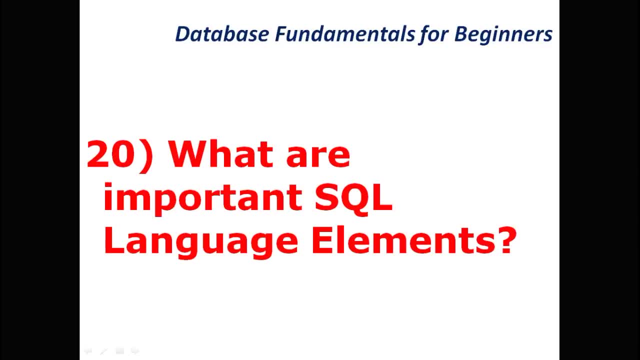 Next Function, functions, Belt in functions. Next Comments, etc. okay statement. next loop, statements for loop while loop, etc. No control flow in SQL, no conditional statements, no loop statements and no branching statements. okay, Thank you.